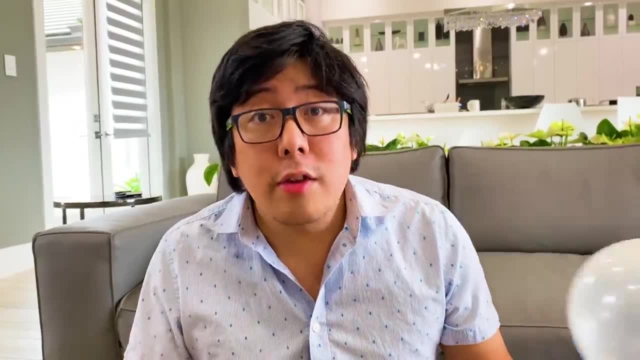 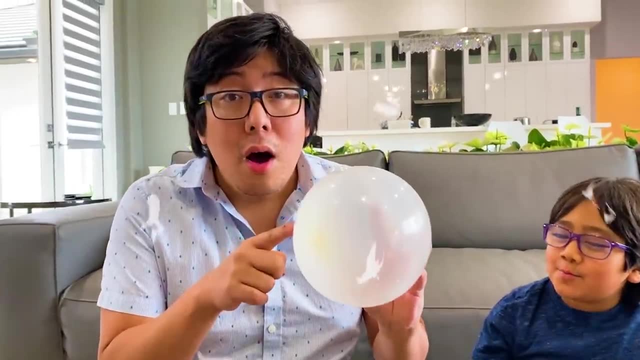 So, guys, if you do this at home, make sure you ask your parents for help. Alright, so today I'm in charge, Ryan, Yeah. So what do you guys think? Do you think the balloon is going to pop or stay the same? 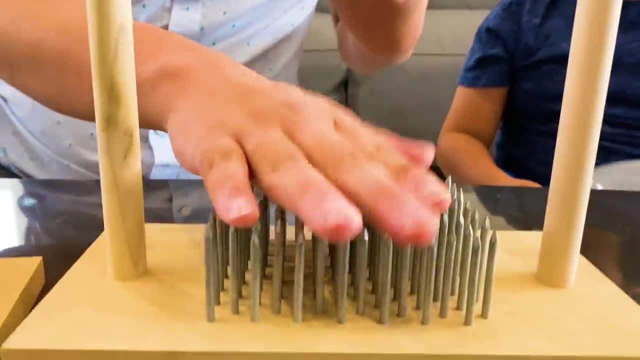 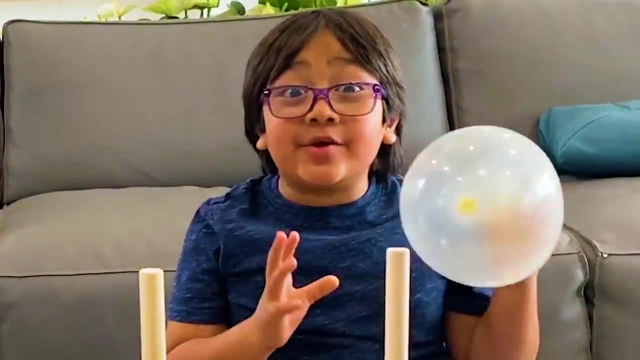 I wonder: Yeah, on top of these nails? Instead of trying it out with a lot of nails, let's do it with one. Let's see what happens. I think it's going to pop if you put a lot of pressure. Alright, let's see what happens. You guys ready? 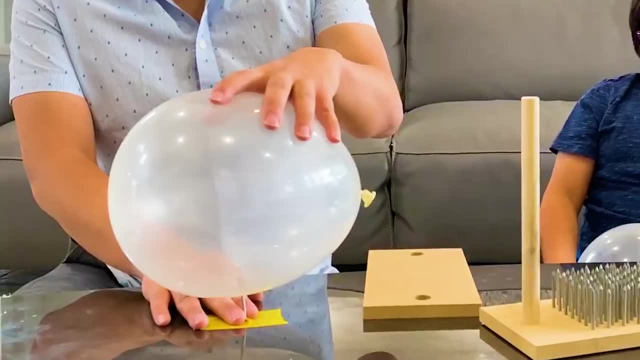 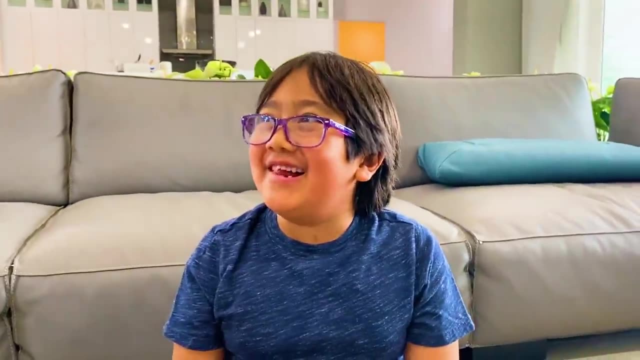 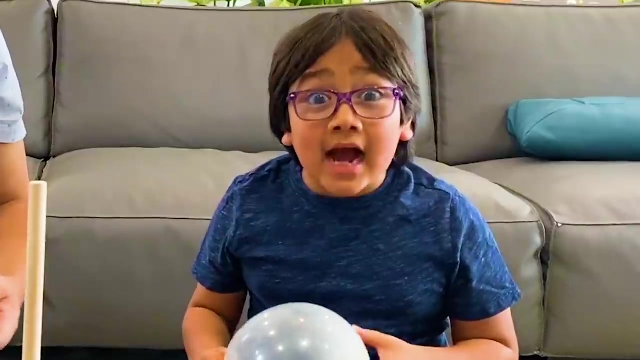 Yeah, Alright, apply the same pressure. It did pop. That was scary, Alright. so, guys, now let's try the same thing with a lot of nails. Yeah, Guys, remember, there are a lot of nails, so remember to ask your grown-up for help. 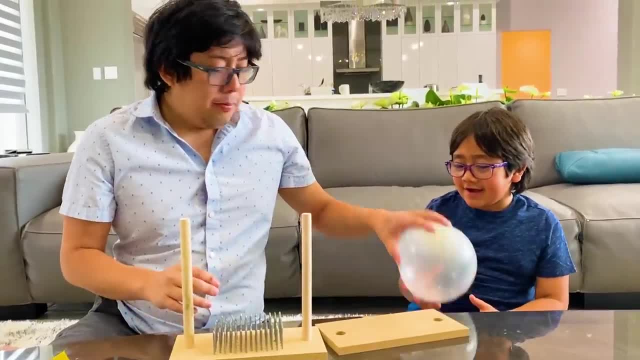 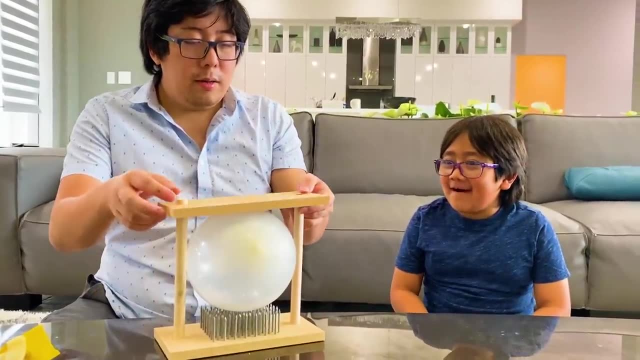 Yeah, because they are pointy right. So you don't want to touch it Here. alright, You guys ready, So set the balloon. I think I know what's going to happen. I'm going to use this board so it won't go anywhere, Ready? 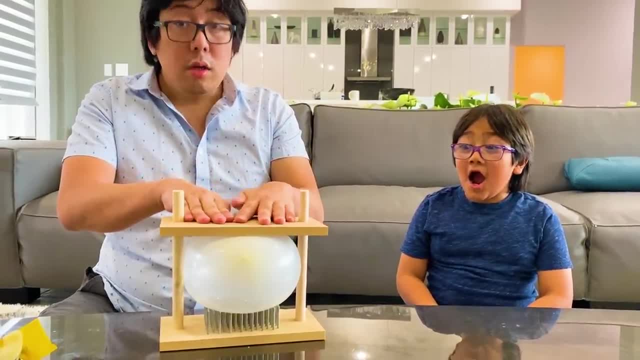 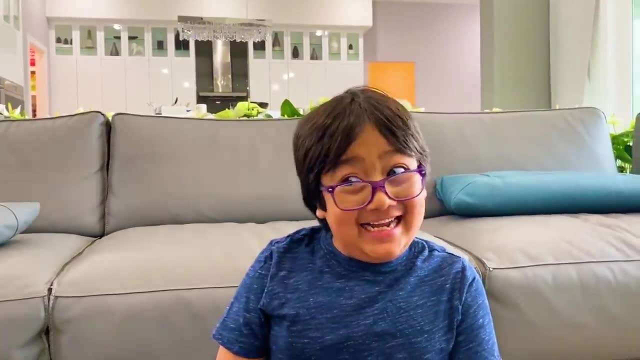 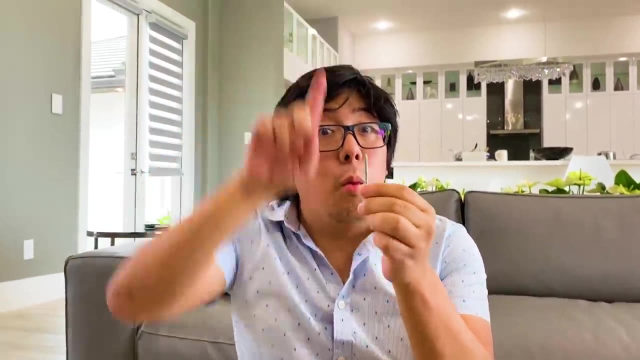 I'm going to press it, Good Guys. I'm pressing really hard, but it's still not popping. You see it? How come there are so many nails, Daddy, but it didn't pop The first time we applied the force into one nail? 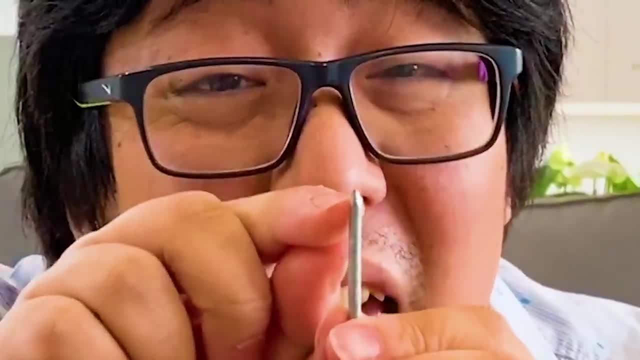 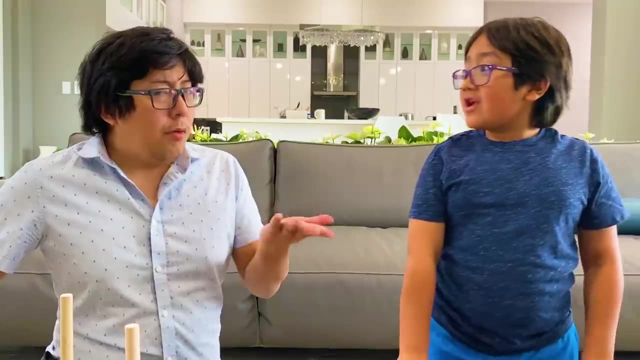 So the area that we applied the force was a very tiny area right here. The second time we applied the same amount of force, but this big of an area. For example, if I press you with my finger, Ow Ow Right. 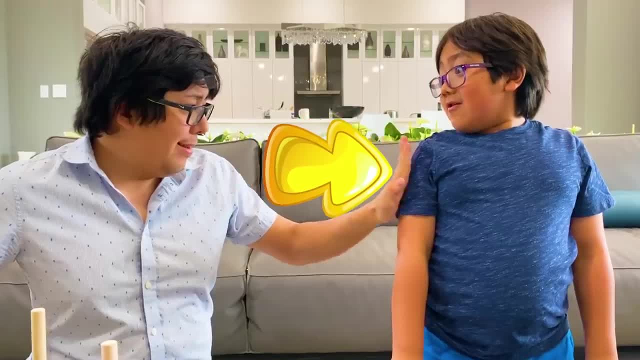 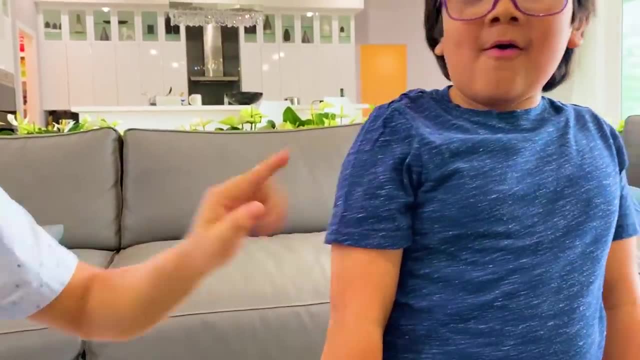 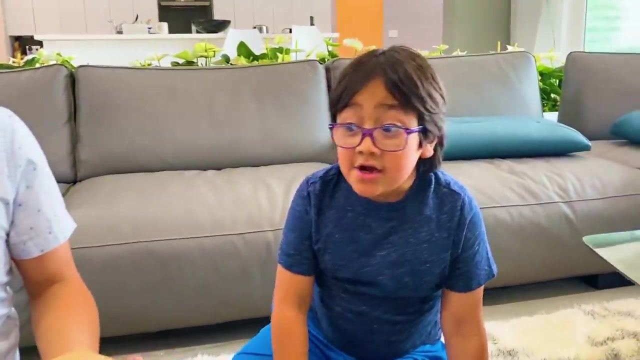 The same amount of force, but if I do it with my palm it doesn't hurt, right? No, But I'm applying the same force but in a different area. Ow See, Ow. But Daddy, can we see how much force it takes to pop the balloon with the giant area? 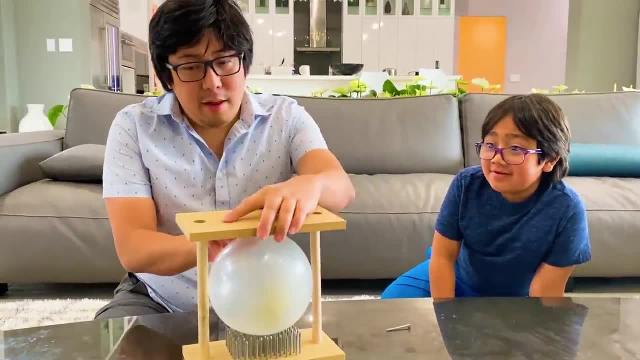 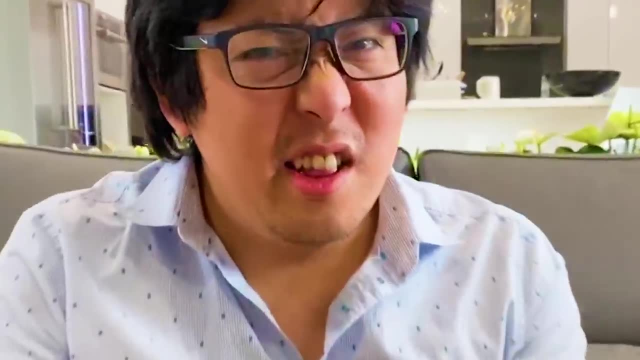 Alright, let's see, Because earlier we couldn't pop it. Daddy, it was like all the way down here. But if I press it with my 100% force, what's going to happen? Are you doing 100%?